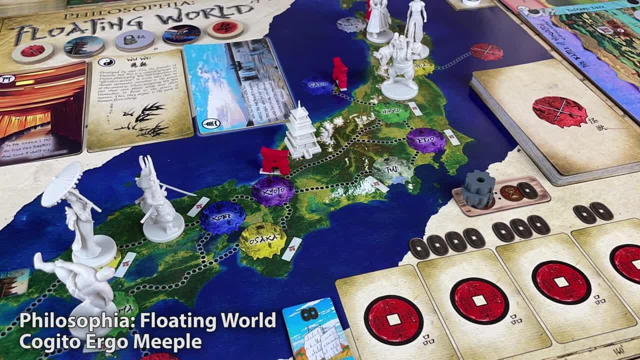 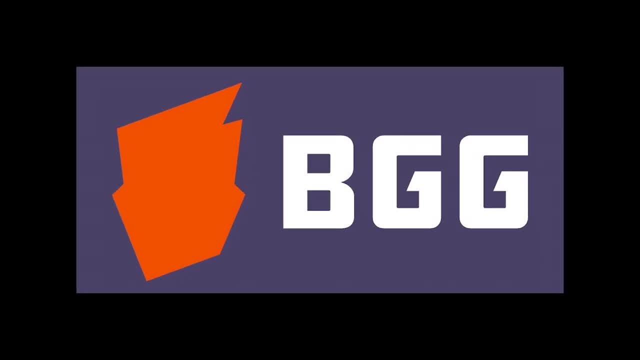 Welcome to Cogito Design, the video series where we take a deep dive into some of the cutting-edge ideas within the tabletop game design industry. The Board Game Geek website has a fantastic list of game mechanics. At the time of writing, this list contains 182. 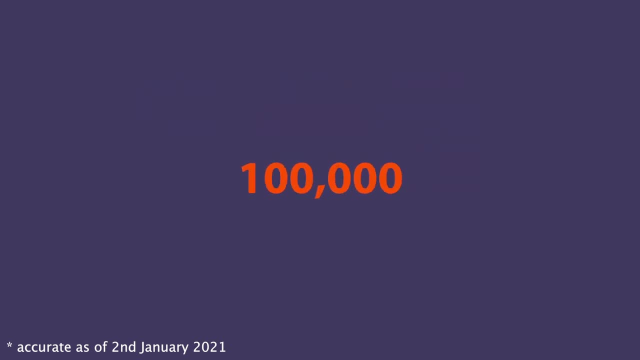 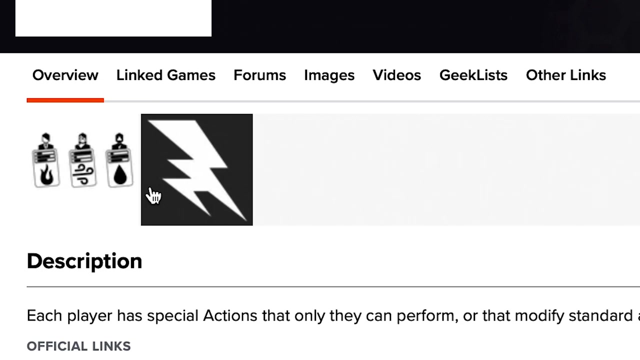 different mechanics that are used in creating the over 100,000 tabletop games listed in their system. When selecting one, you can also see a list of the number of games which use that selected mechanic. For example, there are 2,681 games that utilise worker placement. 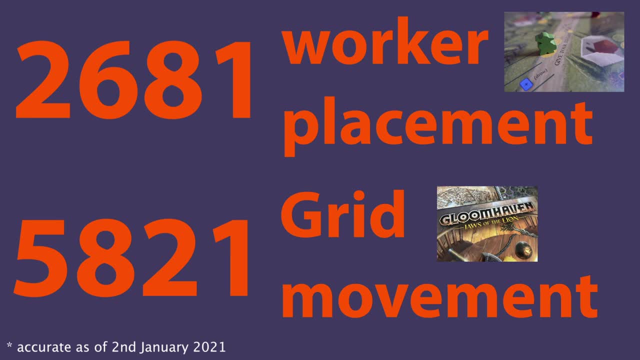 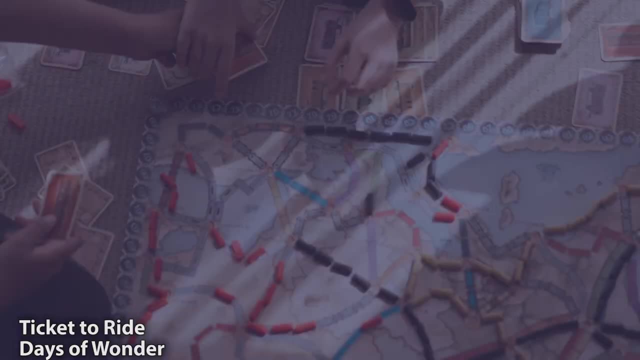 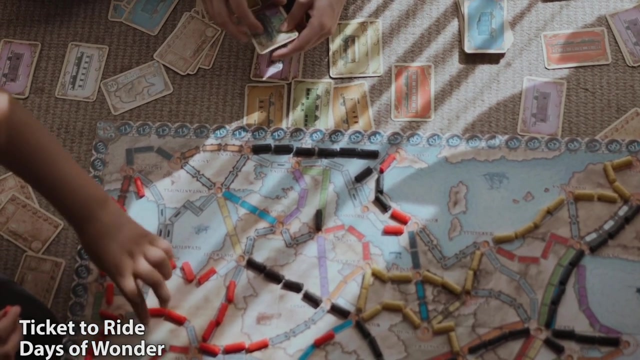 5,821 games that involve movement on a grid and a whopping 13,122 games that have variable player powers. Today I want to talk about one of the mechanics that, in my opinion, is one of the most underrated and underused in the tabletop industry: The old classic. 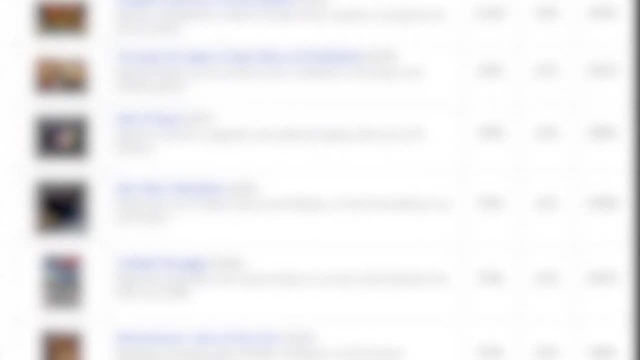 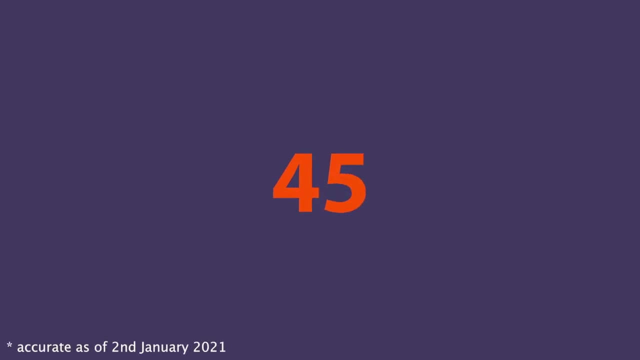 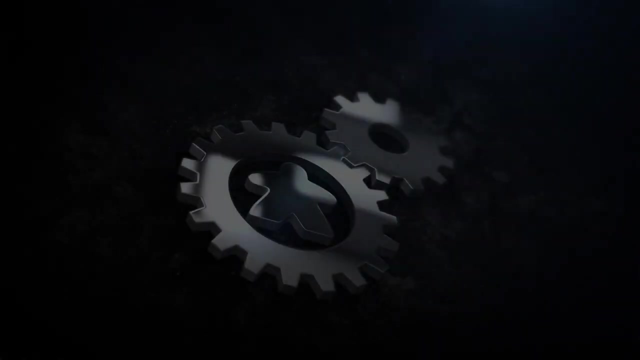 for a millennia. I cut you choose. After over 20 years of accumulating games on the Board Game Geek website, there are still only 45 games in the library that use this mechanic. Let me tell you why you should make number 46.. 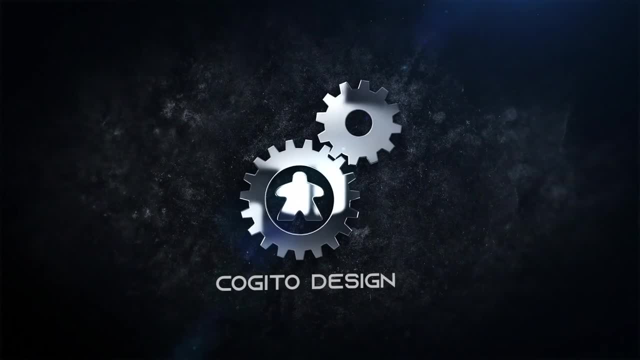 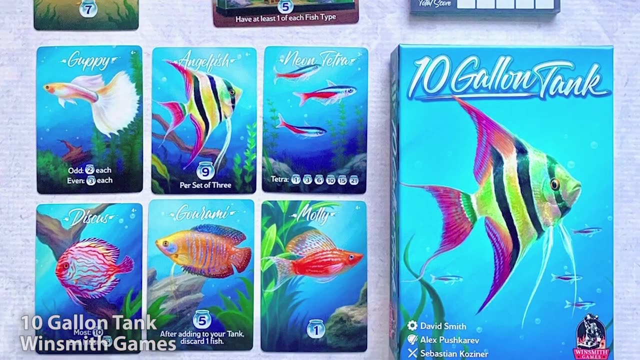 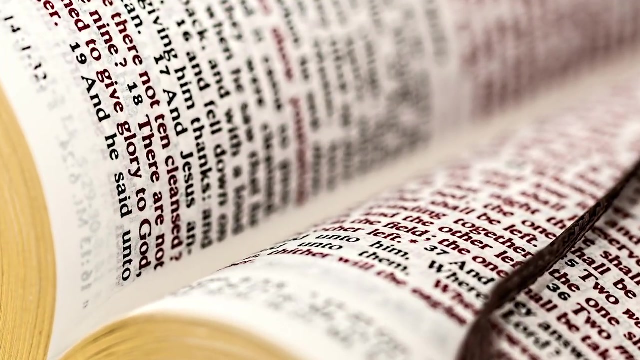 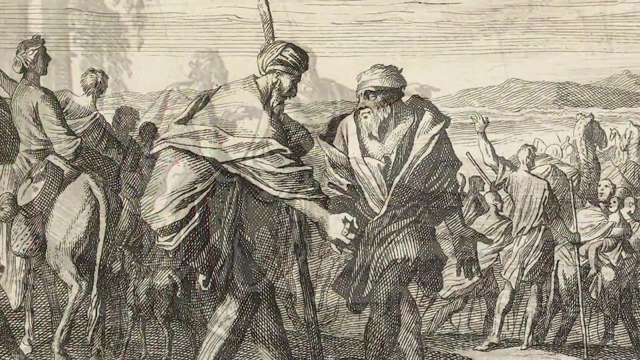 The All Supply Gotta Go, truly ancient. It is even referenced in the Bible, in the book of Genesis, no less. Abraham and Lot both decide to divide up the land of Canaan amongst them. Abraham, being wise, draws a line through the land as equally as he can and then allows Lot to pick either the east or the west. 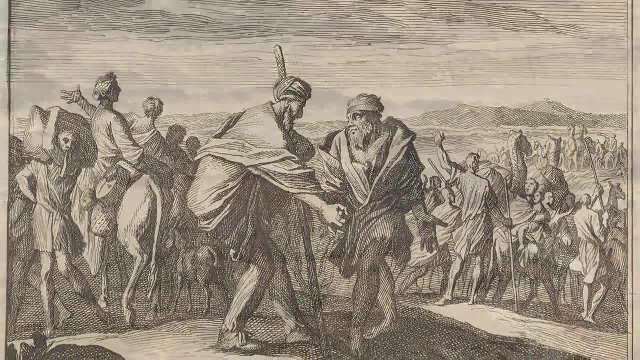 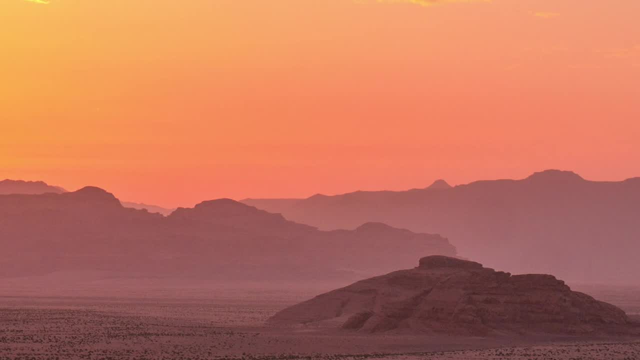 of that line. This removes all possibility of envy, as Abraham is incentivized to draw the line evenly so that no matter what side Lot chooses, the other is just as good. Lot himself is happy because he gets to choose from either portion, so can go for the one he thinks is best In this. 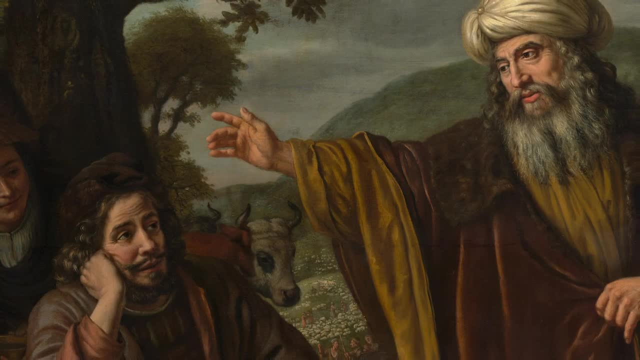 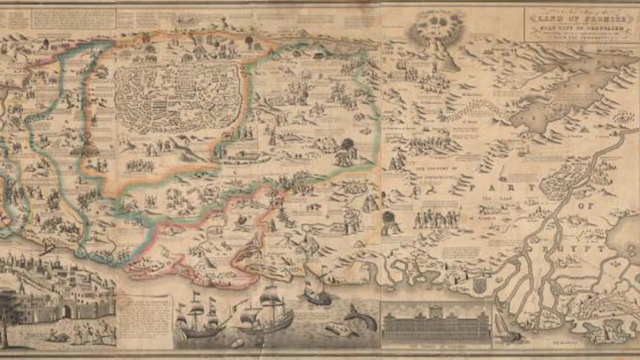 case, the compromise works well, with both living happily ever after. Abraham settles in the western portion with places like Hebron and Shechem, and Lot and his wife settle the eastern portion with towns like Sodom and Gomorrah. Maybe it didn't work out so well for Lot, actually particularly. 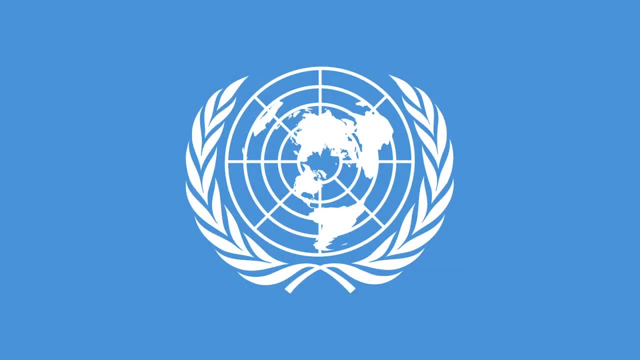 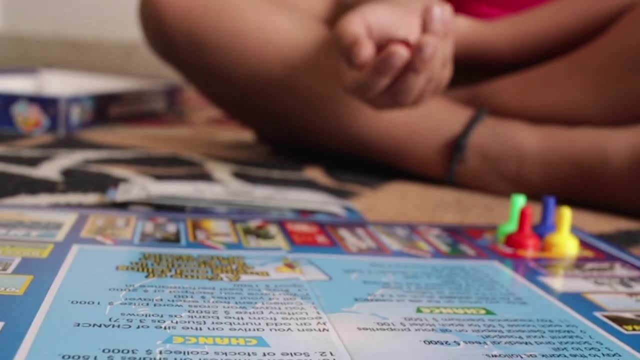 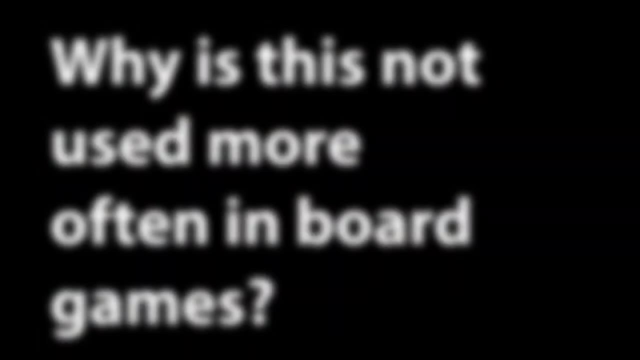 his poor salty wife. More recently, the United Nations still uses this mechanism for allocating areas of the ocean among countries. So, as it is so useful in solving disputes and so easy to understand, being part of our cultural consciousness for thousands of years, why is this not used more often in board games? 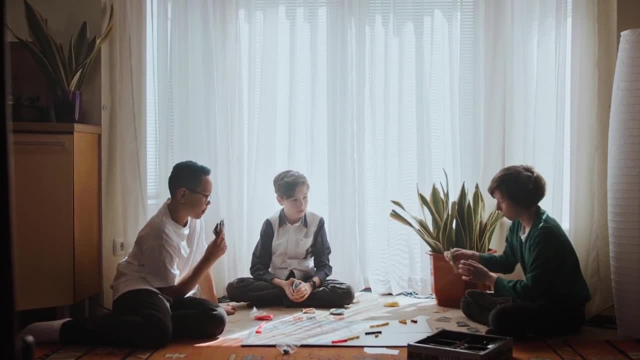 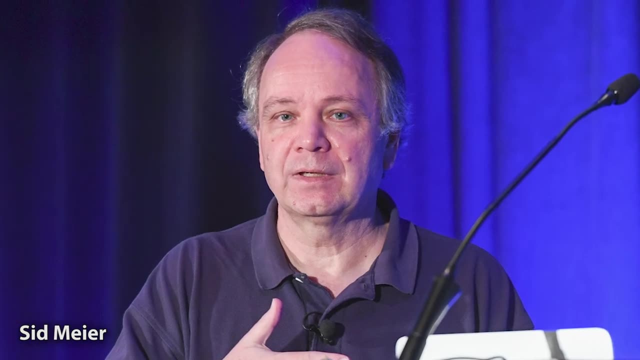 Well, before answering this question, we should first look at some of the reasons why this mechanic is potentially so useful. The legendary game designer Sid Meier once famously said that a game is just a series of interesting decisions. There is probably much more to games than this. 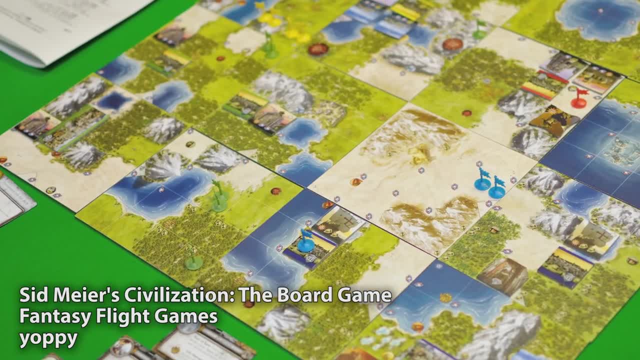 but it is certainly true that interesting decisions are the most important part of a game, and that's exactly what we're going to talk about today. So let's take a look at some of the reasons why these decisions are a crucial part of all good games. 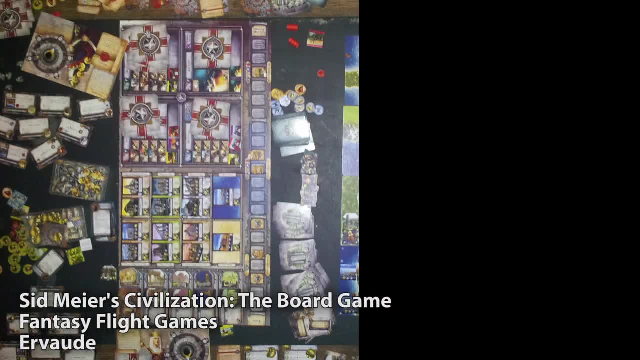 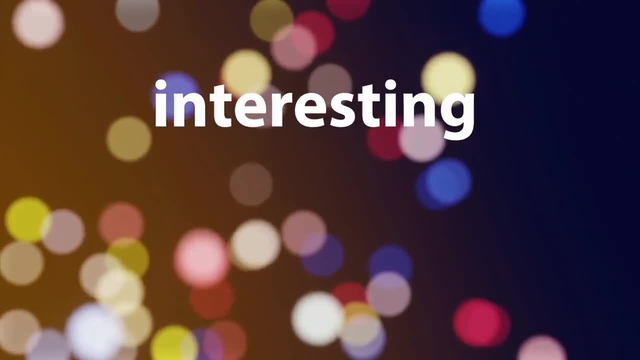 And this is particularly true on the tabletop, where we don't have fabulous triple-A graphics and AI enemies to contend with. iCut You Choose is an excellent and easy way to get some interesting decisions into your game design. To show this, let's look at an example: Hanami Koji by Kota. 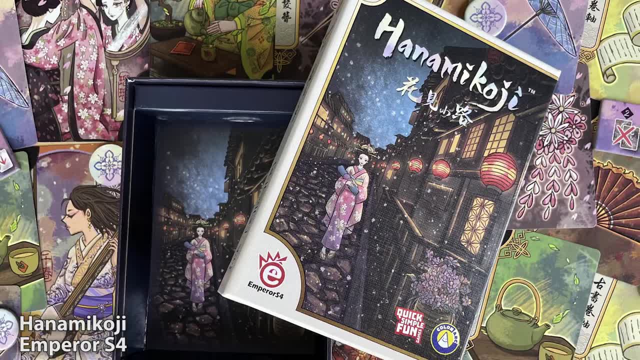 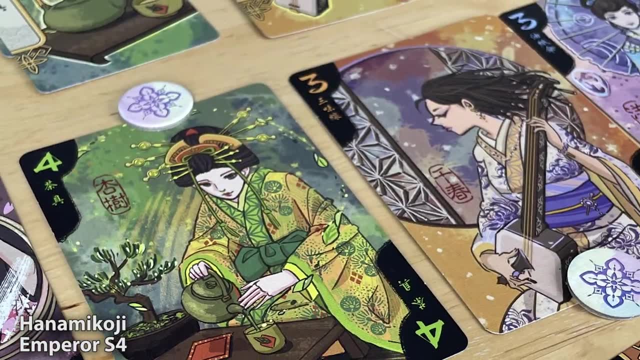 Nakayama. This is a fantastic and simple two-player game which has only four actions but a whole host of juicy decisions to contend with. Two of these four actions involve iCut You Choose, and these are by far the most interesting parts of the game. 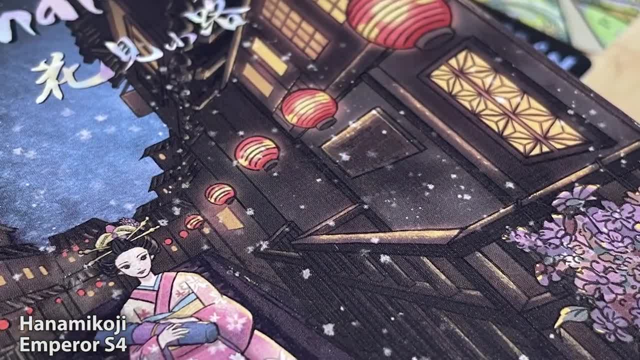 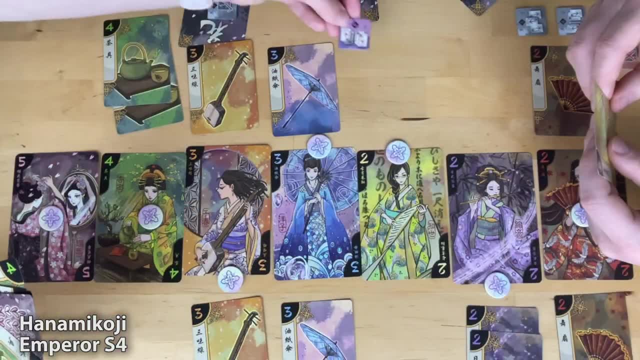 In Hanami Koji, you are all bidding for resources to charm beautiful geishas into your tearoom. This can be easily done, as geishas are apparently easily enticed by trinkets and tea. In one of the actions, you take four of your cards and divide them into two piles. 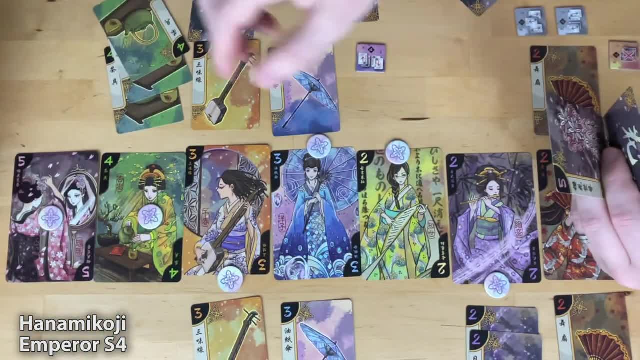 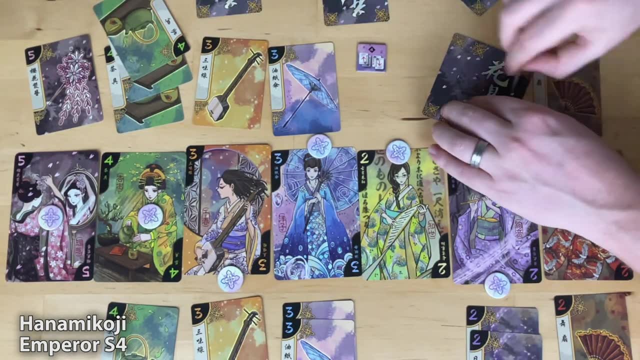 containing two cards each. Your opponent picks one of these and you get the option that remains. This is simple enough, but it actually creates two great moments of tension and decision in the game. Firstly, the act of dividing up the cards itself is an interesting 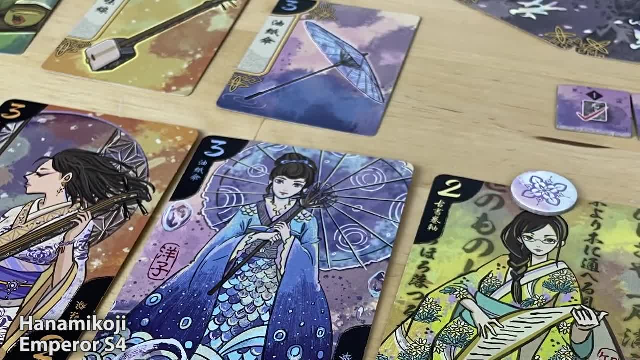 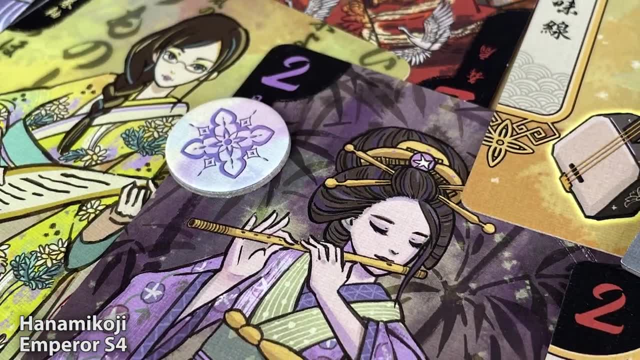 one. All cards in this game are beneficial to players, and so you have to read the game and predict what your opponent will choose when creating these two options. Secondly, of course, your opponent has the decision of which option to choose. This is inevitably an interesting decision. 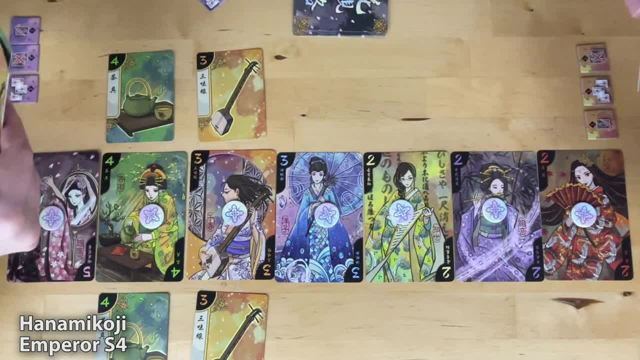 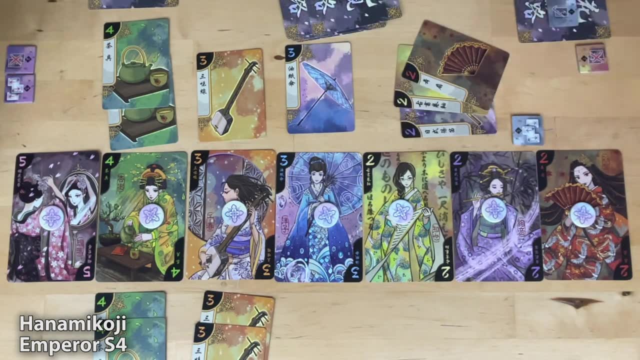 as the mechanics of the game push you to make the two options as even as possible. So, with just one simple mechanic, you have two really interesting decisions using just one need-to-buy card, That is, play it at any time. A kickback with Gemini Cardball token and four. 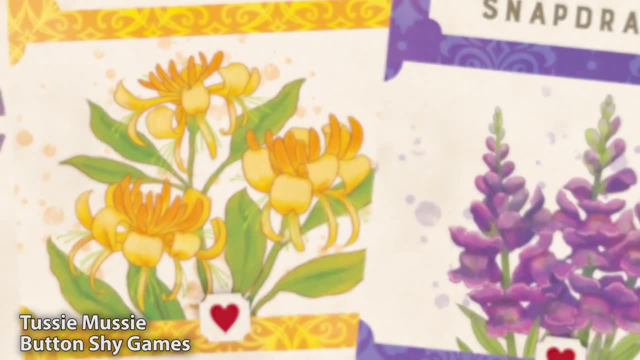 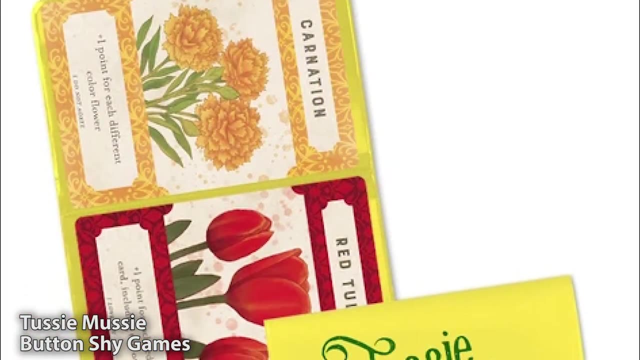 playing cards In terms of sheer efficiency. compare that to the number of components some games need for their interesting decisions. And also there are many different ways to approach the I Cut, You Choose mechanic, Tusy Mussy by wing-span designer Elizabeth Hargrave. 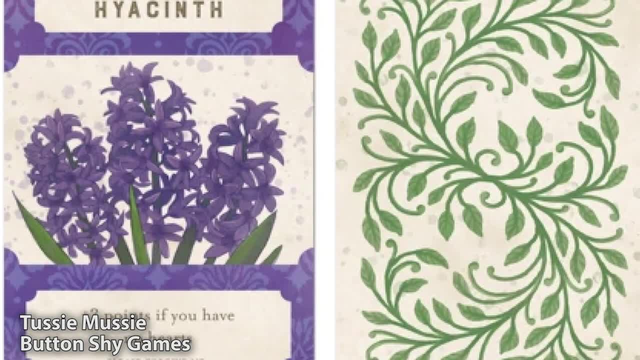 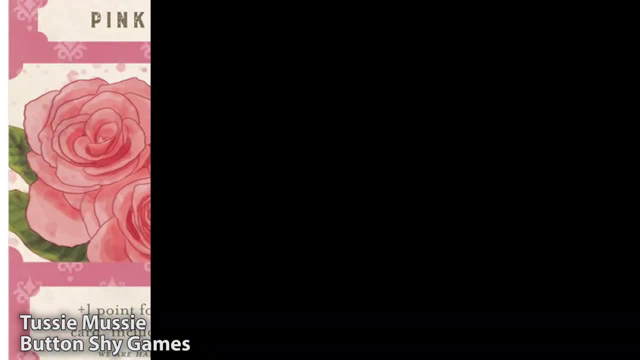 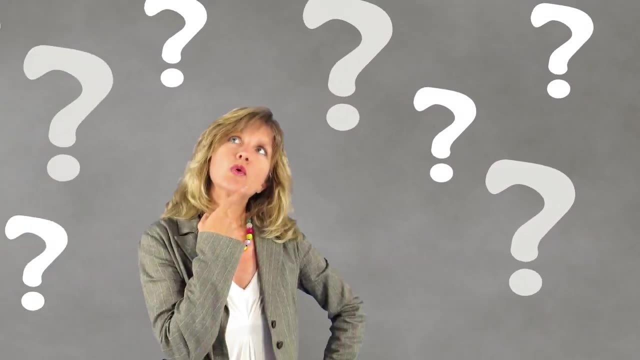 is another interesting example. In this game, players choose two cards. They place one face down, sight unseen. This leads to a really interesting psychological face-off between players. Why have they placed that great card face up? Are they secretly hiding an even more fantastic card face? 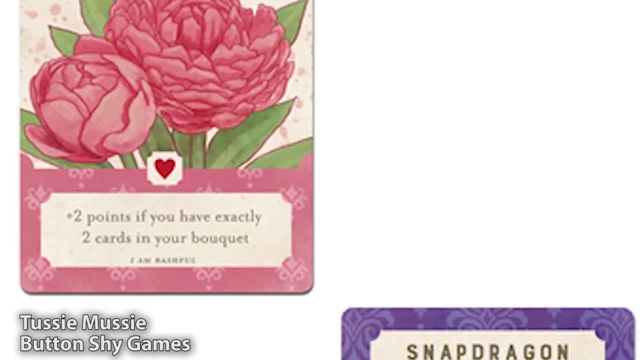 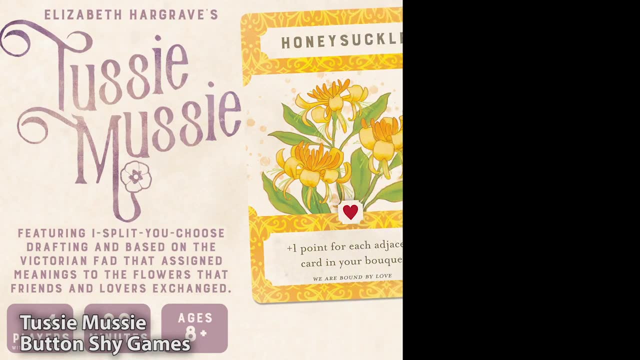 down, Or are they just bluffing? Tussie Mussie creates interesting decisions and satisfying tension, all with minimal resources and rules. And Tussie Mussie does all this with just 18 cards. Another clear advantage of this mechanic is that it can really help increase player interactions. 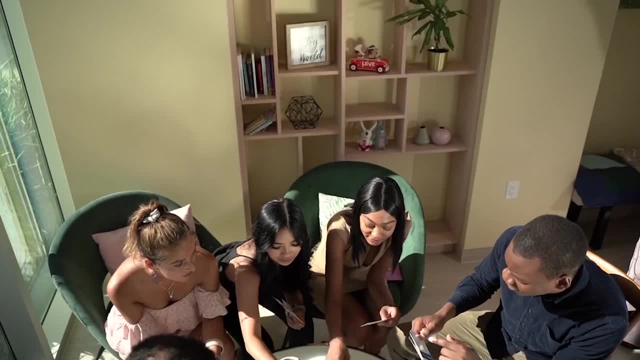 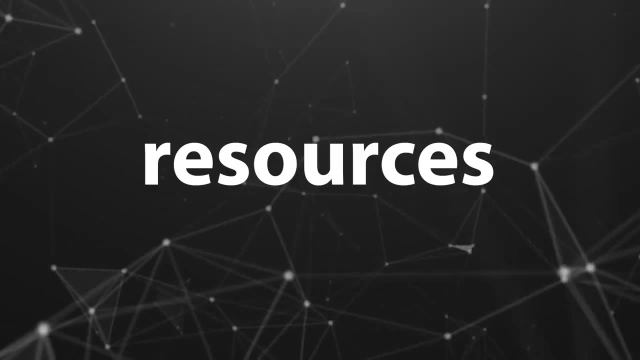 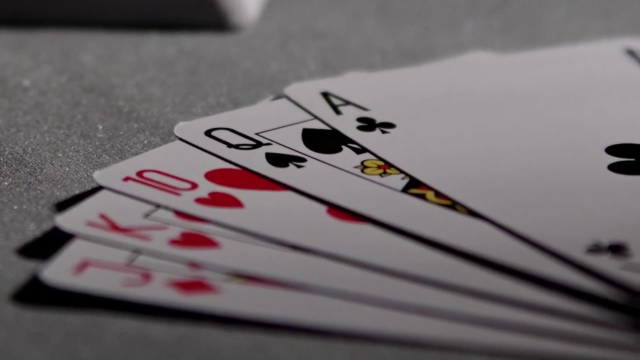 Without these interactions being negative. To divide the piles evenly. in most games you really do need to pay attention and care about what your opponent is doing and what resources they are searching for or path to victory they are focused on. I Cut You Choose can turn a dry game of multiplayer solitaire into something rich and involved, where players 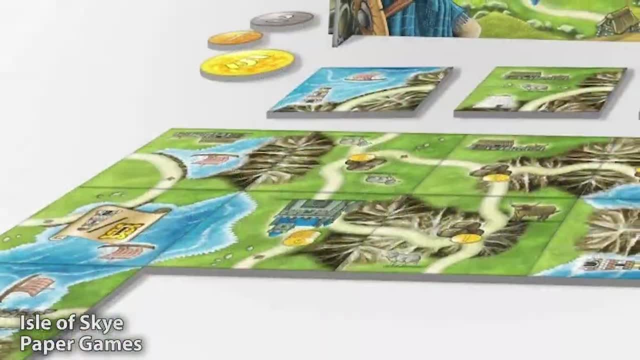 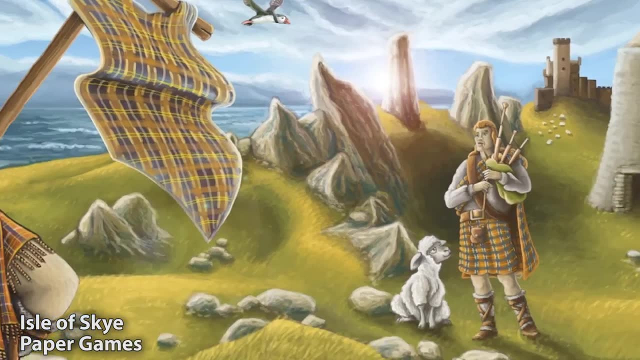 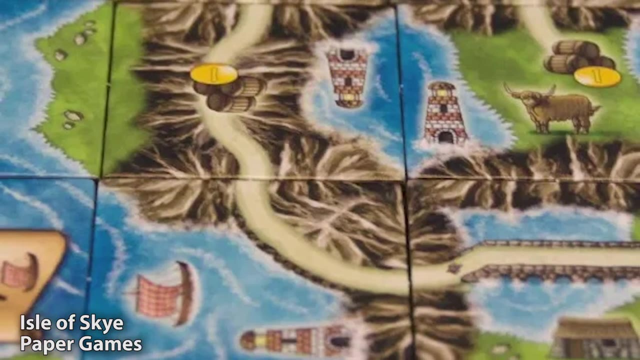 are truly invested in the actions of their opponents. There are also some really interesting variations of this mechanic. In Isle of Skye by Alexander Fister and Andreas Pelikan, we see more of an I Price You Choose mechanic, where players secretly price valuable tiles behind a screen in one phase and then purchase tiles from any of the other. 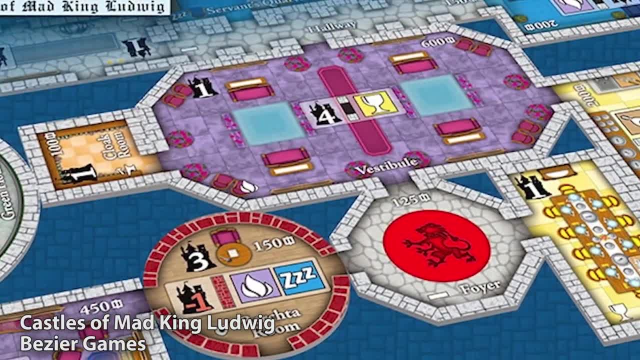 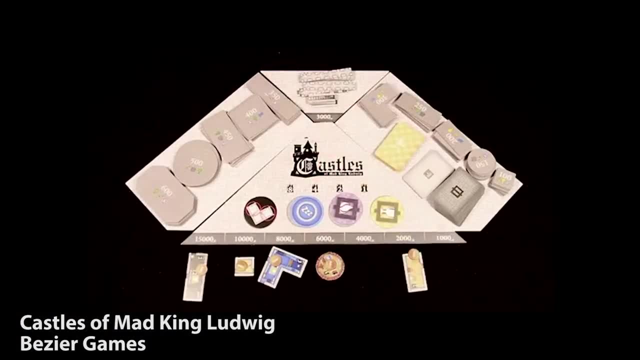 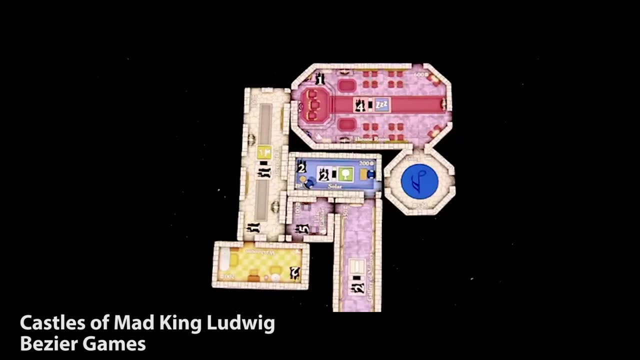 players in the following phase. A similar mechanic is in the classic Castles of Mad King Ludwig by Ted Alsbach. In this game, one player each round takes the role of master builder, setting the prices of all the available castle rooms. The catch is that the master builder can only buy. 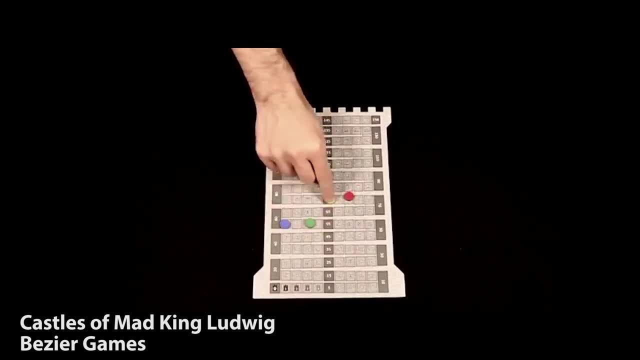 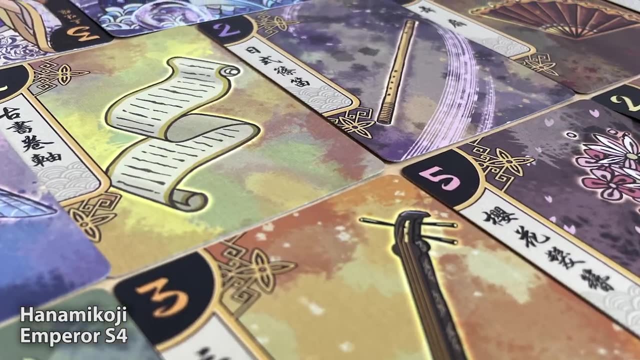 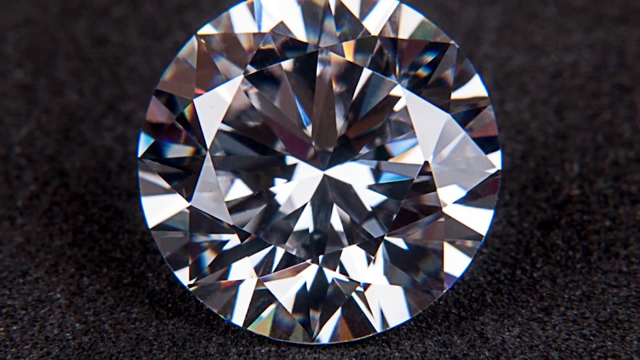 rooms after the other players. In both these games, setting the prices is an interesting decision, and then choosing from these options becomes another interesting decision. Sid Meier would be proud. It's just such a versatile and interesting mechanic With all these clear and obvious benefits, why again has this gem of? 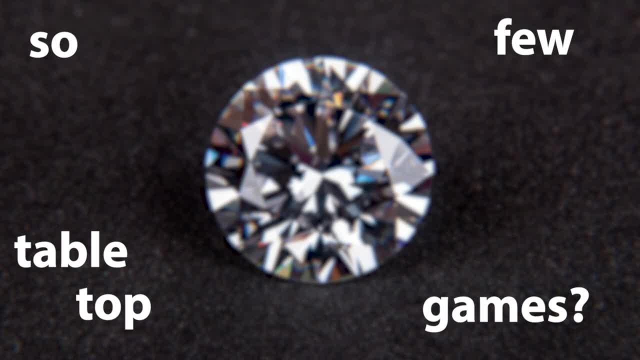 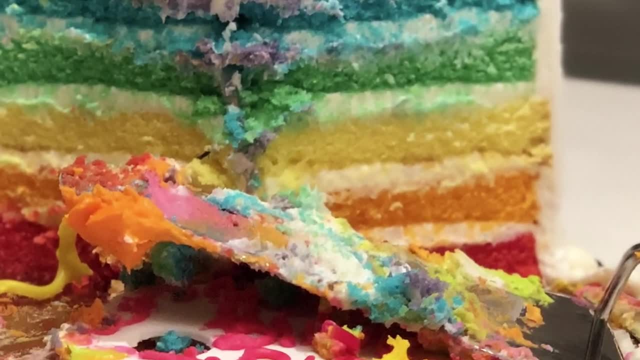 a mechanic made its way into so few tabletop games. Well, there are some reasons for that, but I also think they can be overcome. Firstly, as all people asked to cut the birthday cake in this way know, there is a slight disadvantage to the cutter. 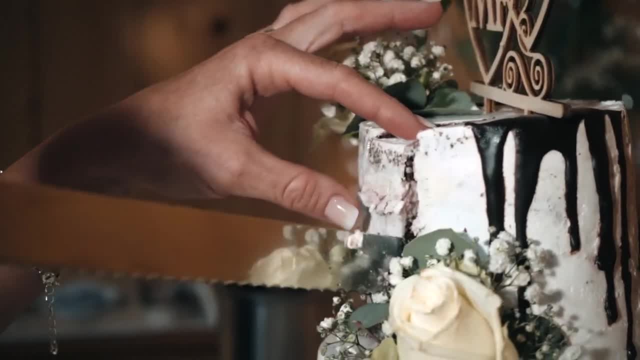 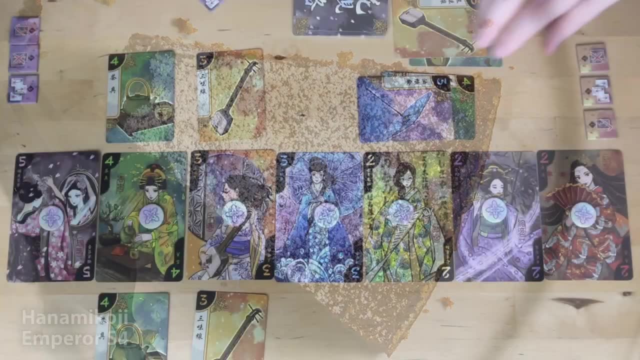 What if the cutting skills aren't up to scratch and you accidentally make one side too big? This disadvantages you, as the chooser will obviously just take the bigger slice. In the Hanami Koji example I gave earlier, it's much better to be the chooser than the cutter. 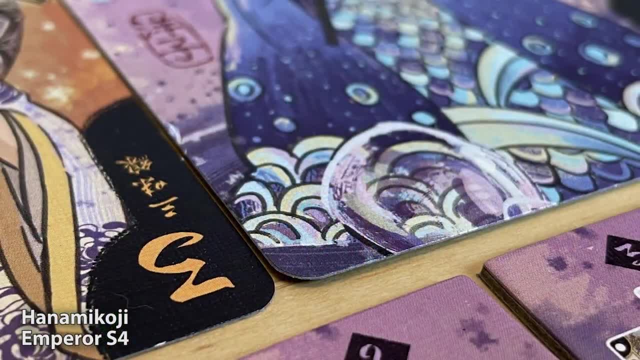 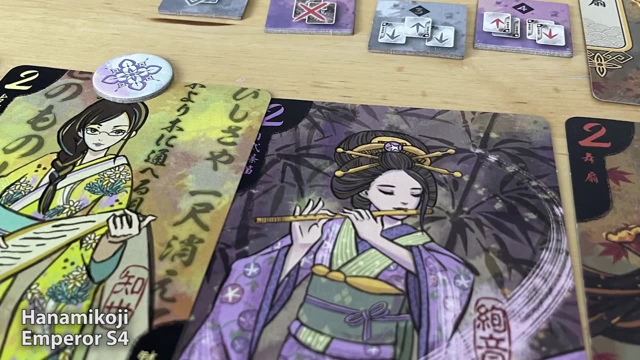 There are, however, several ways to mitigate this in a game. The simplest approach is the one that Hanami Koji itself uses: Simply ask both players to be the cutter and the chooser at different points in the game. This evens out that slight imbalance of power whilst retaining the fun mechanic. 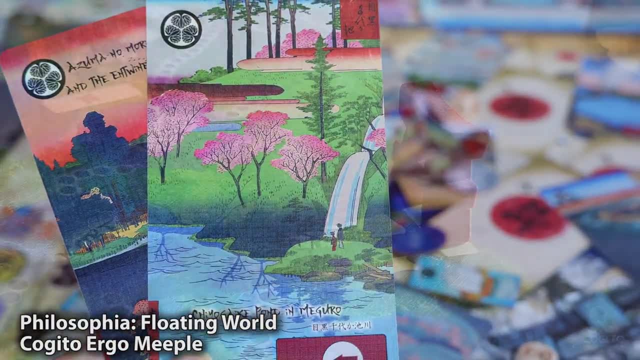 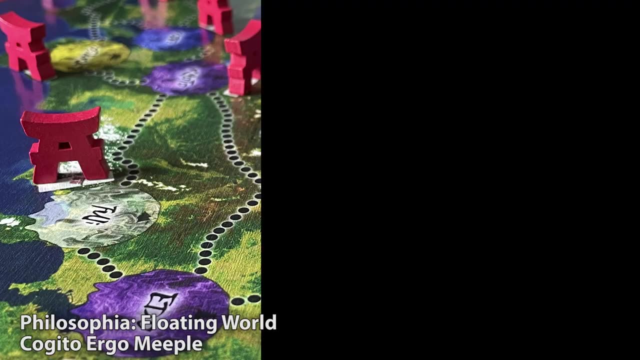 Another approach is to remove the remainder from going to the cutter. This is something that we chose to do in our latest game, Philosophy of Floating World. This game is a fully simultaneous deck builder set in feudal Japan. In Floating World, you draw. 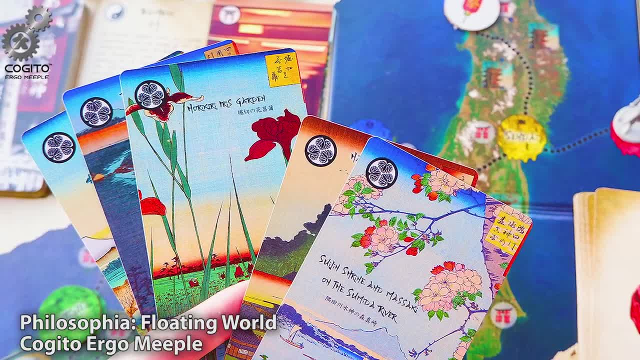 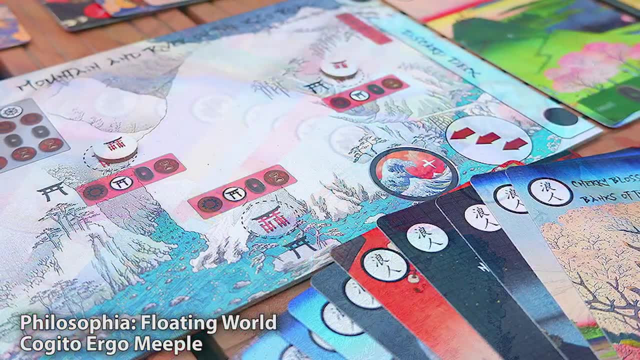 cards from your opponent's deck and then separate them into two piles containing an uneven amount of cards. Your opponent needs to pick one pile and then discard the other. This discarding of the other pile makes a big difference to the gameplay, as the cutter is no longer left with the remaining. 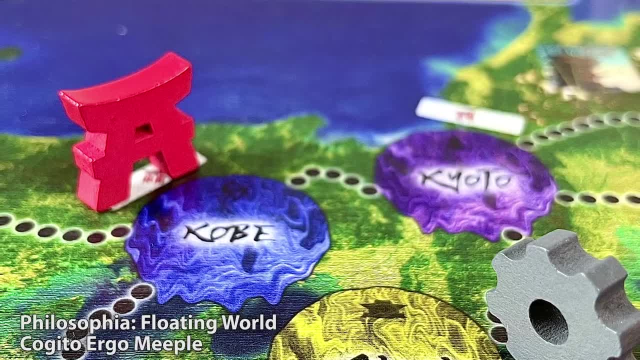 choice, just as it was in the previous game. This means that the opponent will be able to discard the cards themselves, with the addition of the cards, as it is the most satisfying act of dividing the cards. They themselves also get to be the chooser when two piles of cards are returned back to them. 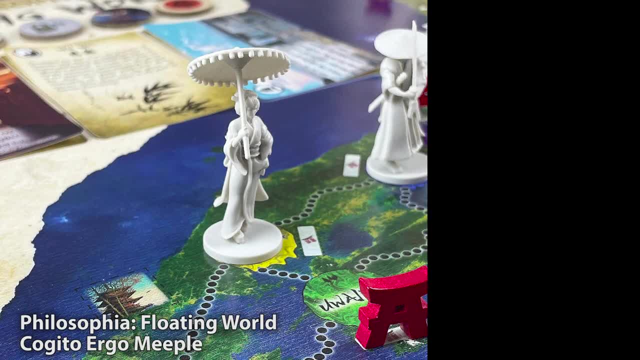 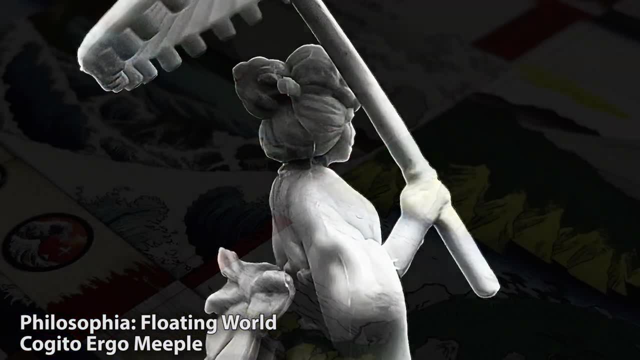 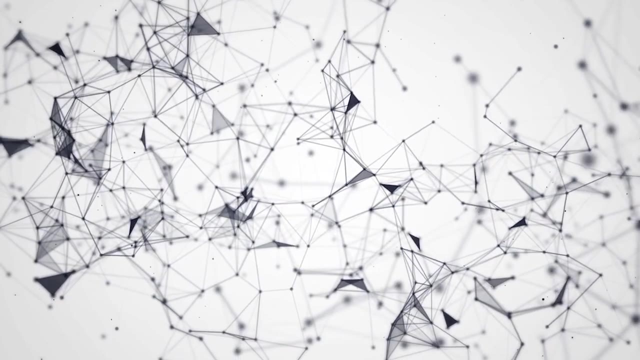 We have been really pleased with the response to this mechanic, as it is interesting and really makes players notice and care about the strategies of the people they are playing with. This approach also has the added benefit of being simultaneous, therefore eliminating player downtime. Another potential issue is that this works best with two players. 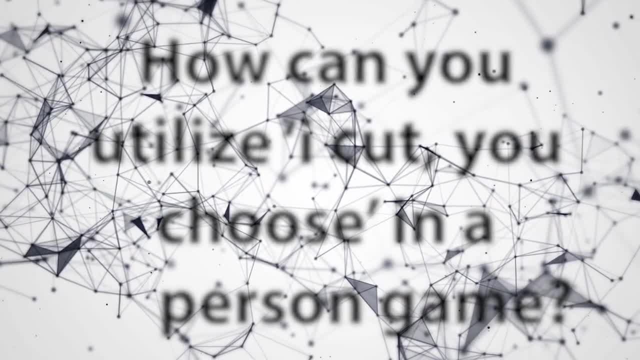 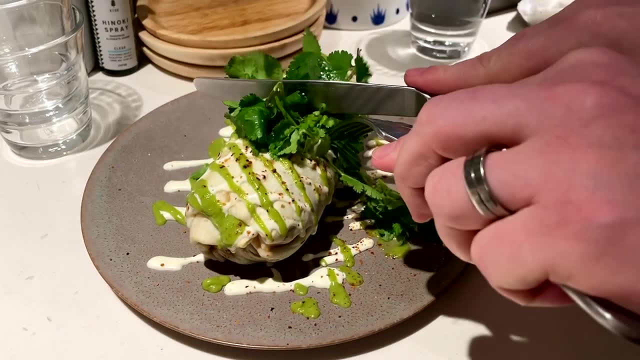 but many games have player counts much higher. How can you utilise iCut You Choose in a three or even a nine person game. This is a tricky issue and in our opinion, it probably does work best if you can keep each of your iCut You Choose interactions to two people. 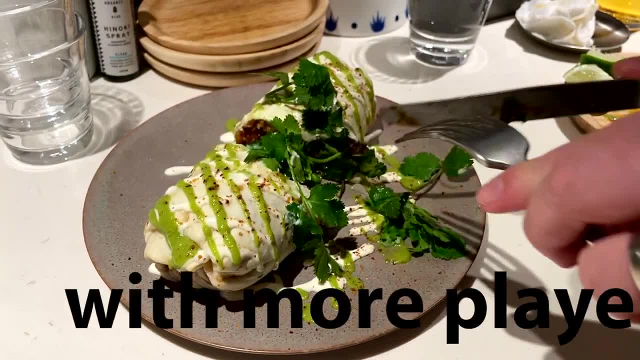 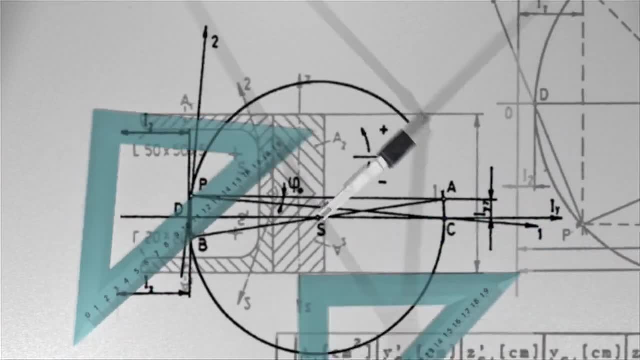 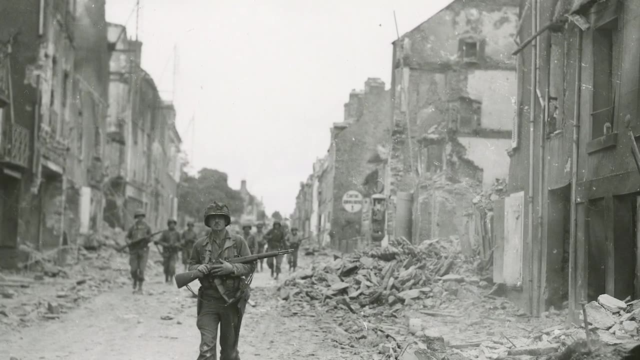 But, that being said, it is certainly not impossible to do well with more players. Interestingly, this problem extends beyond just tabletop games and into the world of pure mathematics. One of the best solutions was provided under very difficult circumstances During the Second World War. the Polish-Jewish mathematician, Hugo Steinhaus, was hiding from the Nazis. 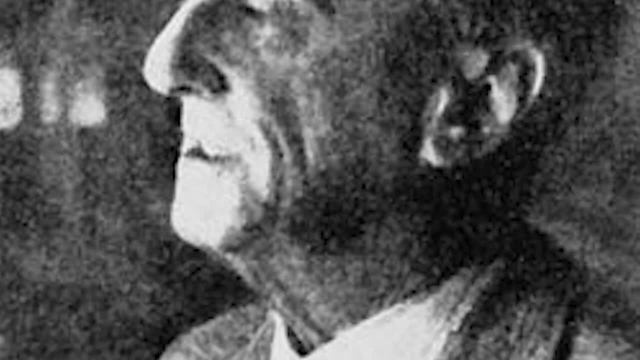 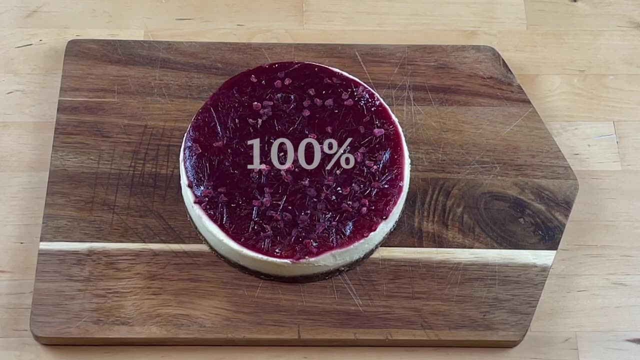 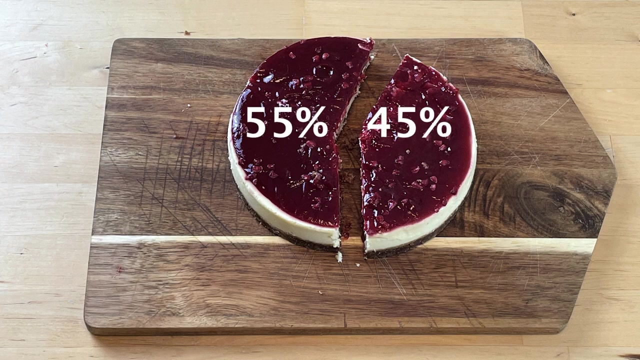 and he used this time in hiding to create a wonderful solution to this problem known as the Last Diminisher. Imagine you are cutting a cake amongst three or more people. The first person cuts a slice, then the second person has a choice: Either allow them to have that slice or cut some amount off the same slice. 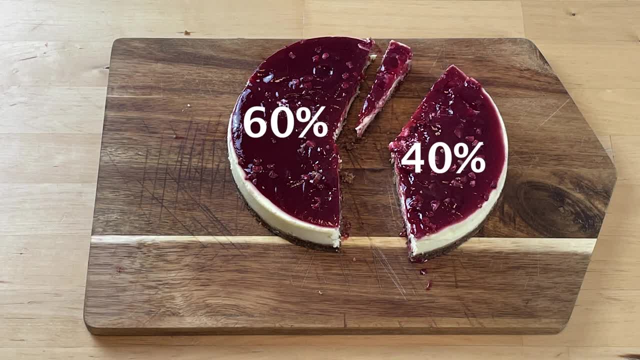 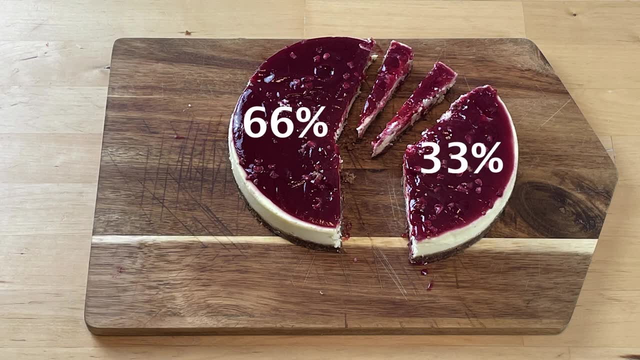 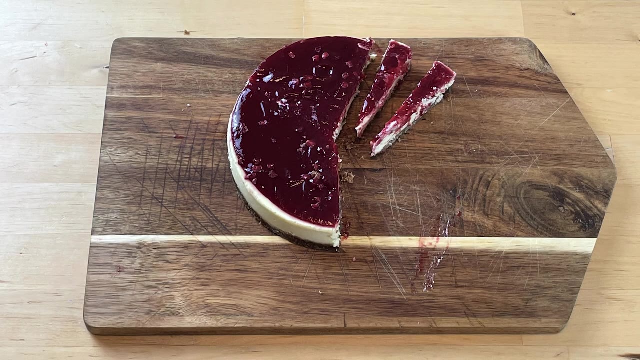 The third person has the same choice: Either allow the second person to have the new, smaller slice or cut more off themselves. This continues until someone decides that the last person who cut the cake did so fairly. They take their slice and the process restarts with the remaining cake eaters. 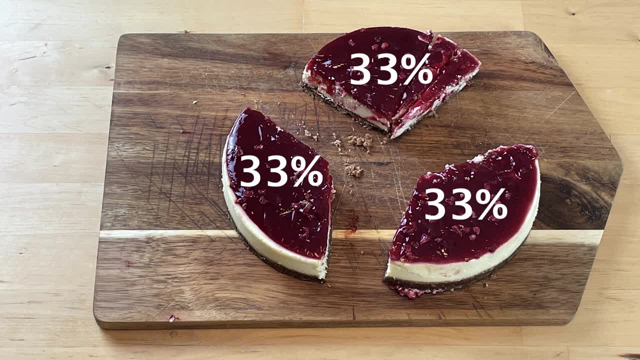 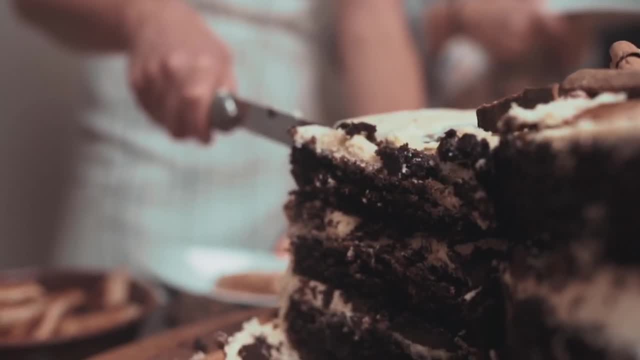 There is no incentive to cut a slice that is smaller than your fair share and no reason to allow a person to take more than theirs, and thus all parties end up with even slices. It's a pretty brilliant solution, but I've yet to see it incorporated into a board game. 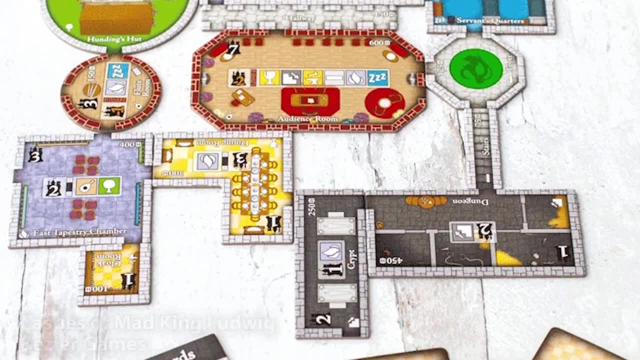 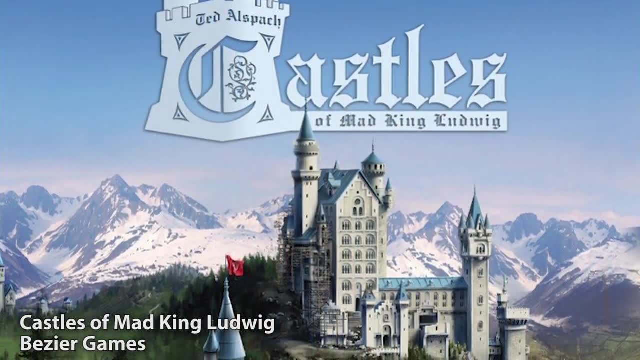 Nor would it keep your cake looking very pretty. Another and potentially simpler way to solve this problem is actually one we mentioned earlier: The I Price You Choose mechanic from Castles of Mad King, Ludwig and from the Isle of Skye. 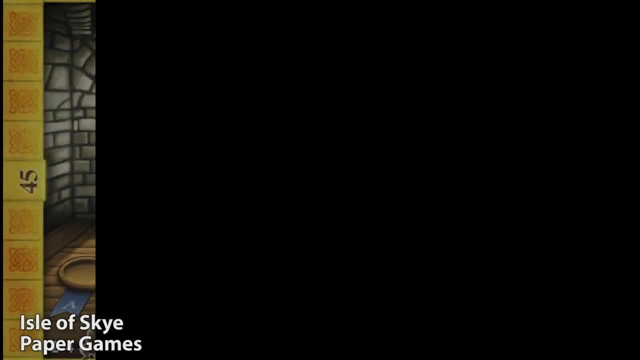 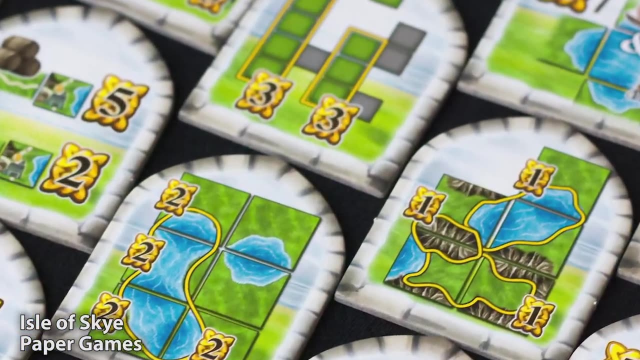 Both have players pricing multiple resources and then creating a marketplace of many choices which allows meaningful decisions for a wider number of players. If players create enough choices, then you will have a host of interesting decisions. This works particularly well if the players have a number of choices to choose from. 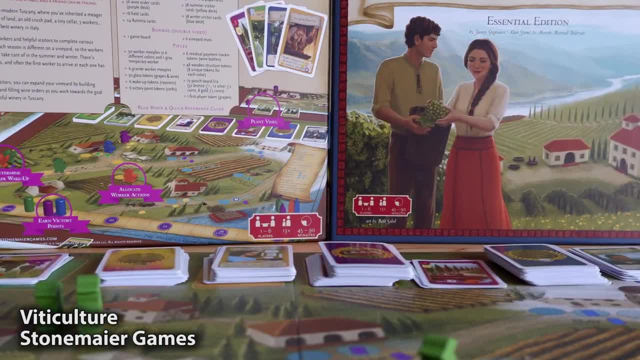 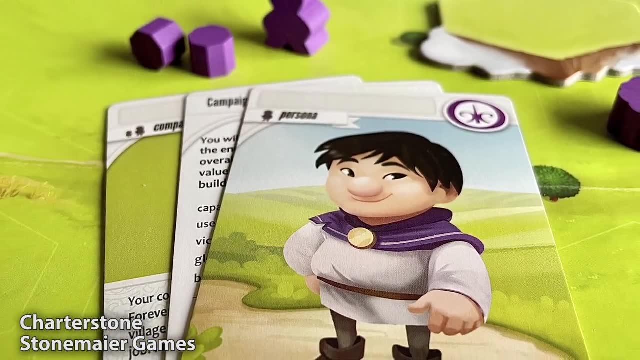 and a number of choices to choose from. This works particularly well if the players have a number of choices to choose from, enough information to make an informed decision, but not so much that they know everything. A final potential issue with this mechanic was given by Stonemaier Games owner and legendary 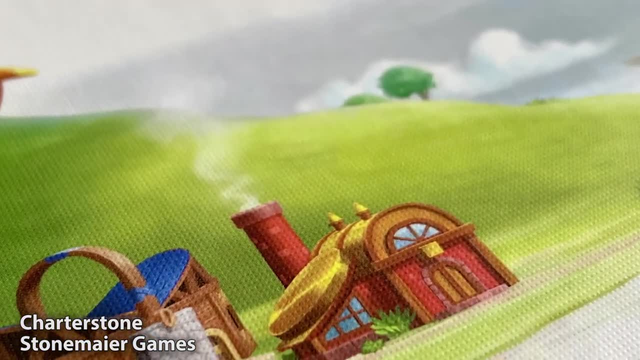 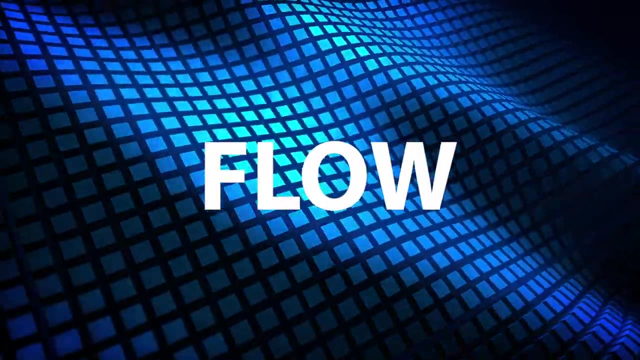 game designer Jamie Stegmaier. He prefers to avoid having distinct rounds or phases in his games, as this helps players achieve what he terms as flow, where play is not broken up but continuously progresses from player to player until the game ends. This can certainly